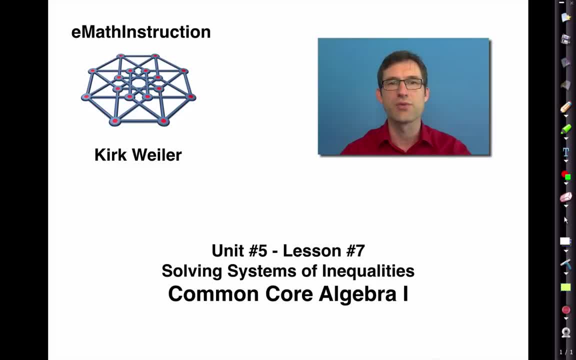 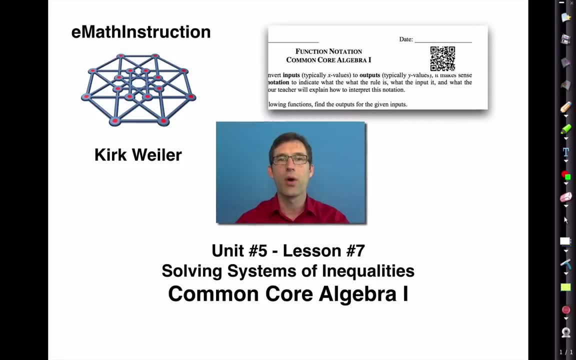 with this video along with a homework assignment, by clicking on the video's description or by visiting our website at wwwemathinstructioncom As well. don't forget about the QR codes on the top of every worksheet. Use your smartphone or tablet to scan those codes and bring you. 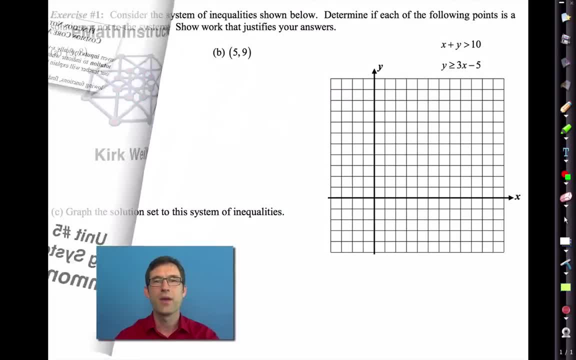 right to these videos, Okay, So previously we've learned about systems of equations and systems of inequalities. We've also learned about how to graph linear inequalities into variables. Today, what we're going to be doing is combining all of those to graph the. 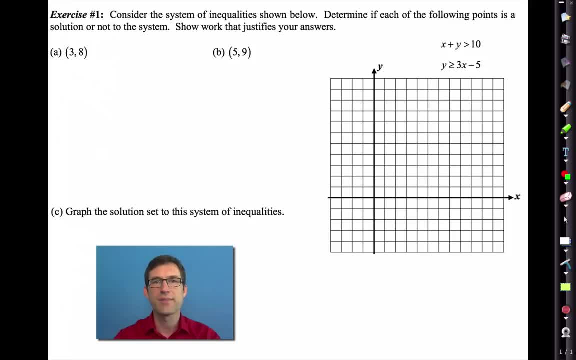 solution sets of systems of inequalities. But first let's jump in in Exercise 1. Take a look at a system of inequalities and try to figure out whether particular points are solutions to those systems. So what we want to do is we want to figure out if the point 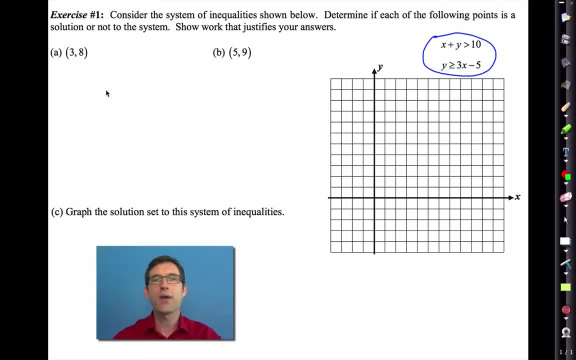 is a solution to that system. Now, it doesn't matter whether it's a system of equality or a system of inequalities or a mixed-up system. The plain fact is: point is a solution to a system if it makes all the equations or 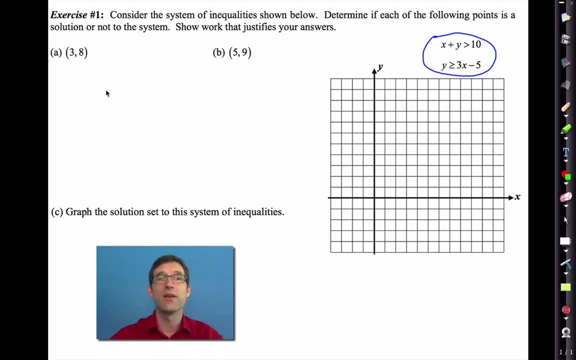 in this case inequalities, true. So let's take a look in letter A. If I take that first, inequality X plus Y is greater than 10, and I put 3 in for X and I put 8 in for Y, right? 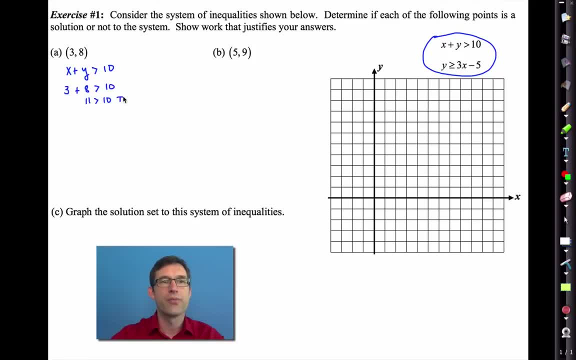 I'll get: 11 is greater than 10, and that's true. If I take the next one, Y is greater than or equal to 3x. question in: oblige, I'll get 8 plus 5, is true. Now, this same inequality. 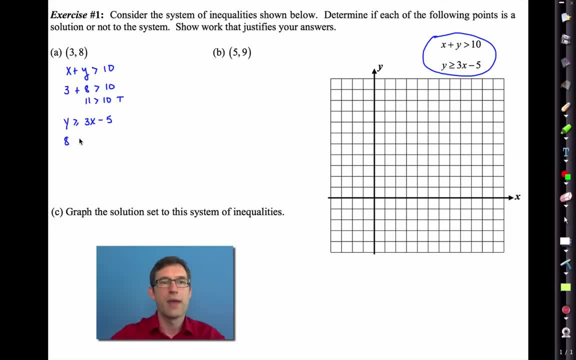 I'll put here: 8 equals 10, which of course makes all 5 parts equal right. But we've 3x minus 5, and I put 8 in for y and I put 3 in for x, I'll get: 8 is greater than or. 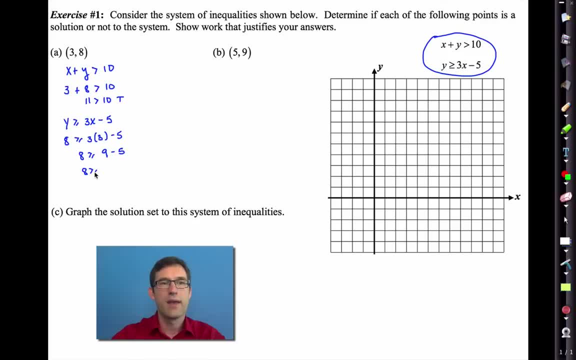 equal to 9 minus 5, 8 is greater than or equal to 4,- that's also true, Because I have those two trues- the answer is yes. So at the end of the day, in letter C, we're going to graph the solution set to this system. 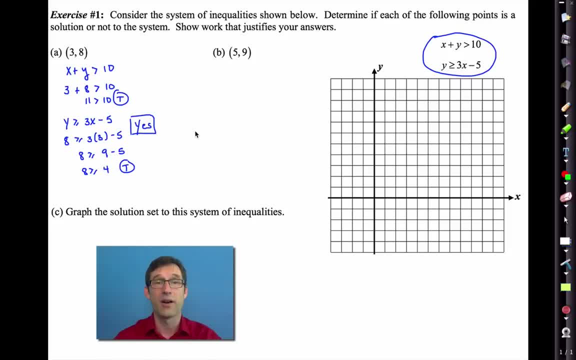 of inequalities, 3 comma 8, better be in there. Why don't you pause the video and see if the point 5 comma 9 is a solution to this system of inequalities? Alright, let's go through it. Hopefully, this time you found that the answer was no, but let's take a look. 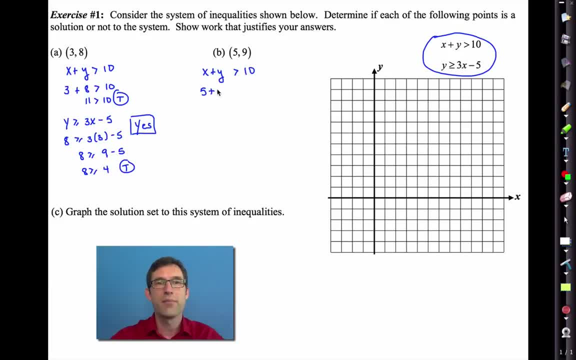 I have x plus y is greater than 10, so I'll put 5 plus 9 in there. greater than 10, 14 is greater than 10, that's true. Okay, Let's try this one: y is greater than or equal to 3x minus 5, so I'll put 9 in there. 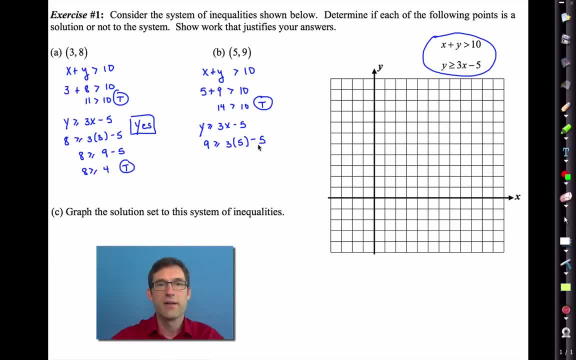 and I'll put 5 in there. 3 times 5 is 15, minus 5,, 9 is greater than or equal to 10, and that's false. Now it doesn't particularly matter that this one's true. the plain fact is, if any of them, 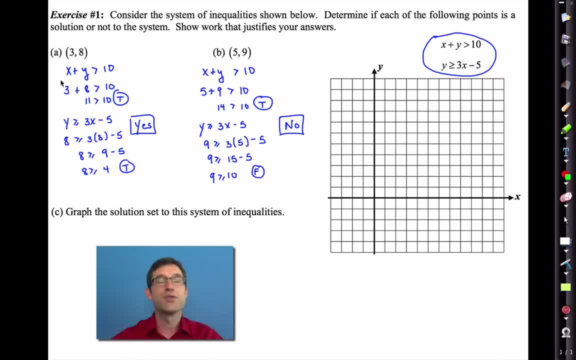 are false. the answer is no. So, just as we pointed out in letter A, When we ultimately graph this thing, that point shouldn't be in the solution set. So let's remember how to graph inequalities, and actually I'm going to start with this. 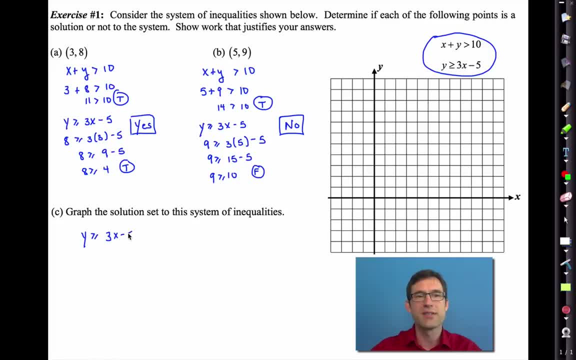 one, y is greater than or equal to 3x minus 5, because it's the easier one. Remember, what we're going to do is we're actually going to first graph this equation: y equals 3x minus 5.. That should be pretty easy, right. 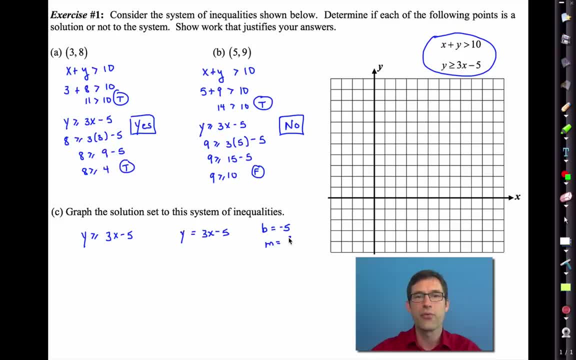 We have a y intercept of negative 5, and we have a slope of 3 over 1.. So 1,, 2, 3., 4,, 5,. all the way down here We're going to go up 3 and to the right 1,, up 3 to the right 1,, et cetera. 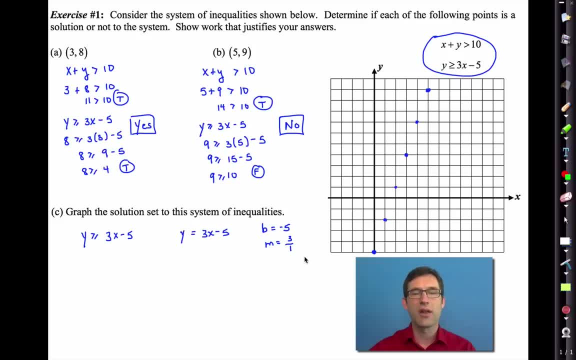 Now we have to make a decision whether or not we then connect these with a dashed line or a solid line. Do you remember how that works? Hopefully, If there's an equal sign here, which there is, then we graph it with a solid line. 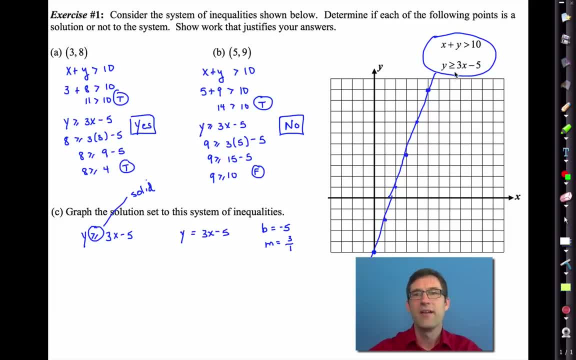 Not my best solid line And we label it with its equation: y equals 3x minus 5.. The reason I wanted to do that one first was because the y was already isolated. In this one there's a little bit more of a challenge because the y is not alone. 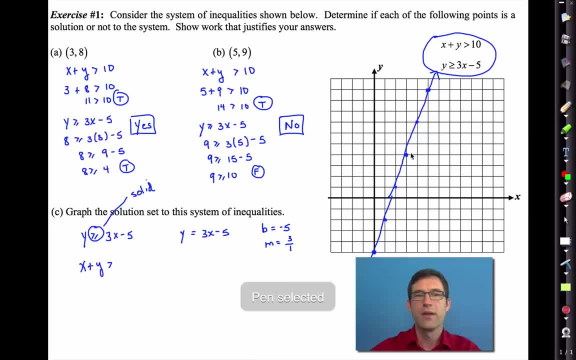 I don't know why I put the equal sign in there. it's not there. X plus y is greater than 10.. Now, that's not a problem. I can subtract x from both sides. Now, remember, a property of inequality is that you can add or subtract anything you. 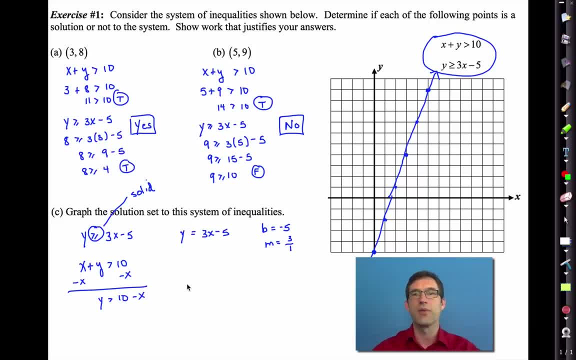 want from each side, and it's not going to change that inequality symbol. That inequality is only going to flip if we divide by a negative. Now what we want to do is we want to graph: y equals 10 minus x, In this case, that b is 10, and that m is negative, 1 over 1.. 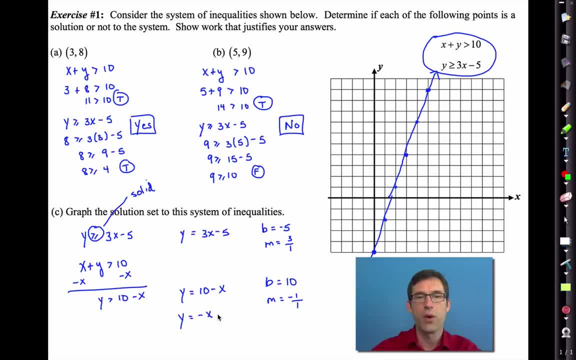 Now, how do I know that? Because I can use the calculator. I can use the commutative property of equality- sorry, just the commutative property of addition- to flip-flop that 10 minus x and make it into negative x plus 10.. 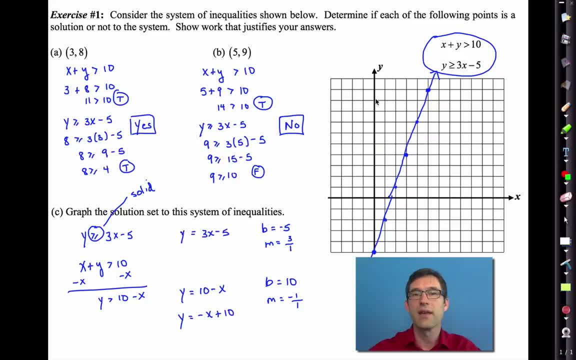 So here we go: 1,, 2,, 3,, 4,, 5,, 6,, 7,, 8,, 9,, 10.. Down one to the right one, et cetera, All right. So that's the commutative property of addition. 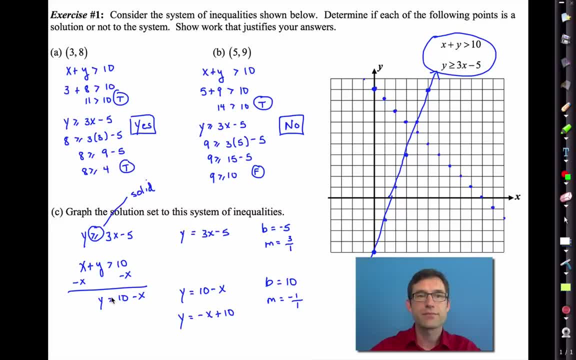 All right. Now in this case, though right in this case- since there is no equal sign, we need to draw this in dashed, All right, But now we've got some shading, okay. In the first one it was: y is greater than or equal to 3x plus 5.. 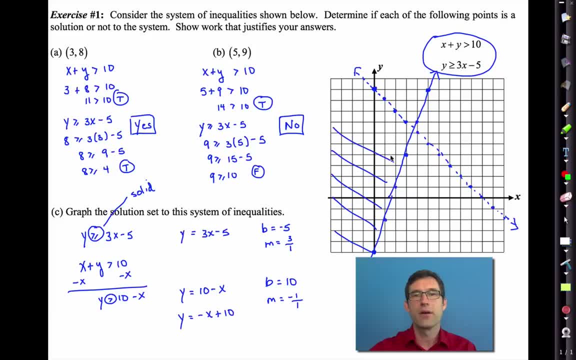 So we're going to shade above, above, 3x plus 5.. All right, All right, Above this line, And actually I'm going to change my color to red for the other one. The other one was also greater than. 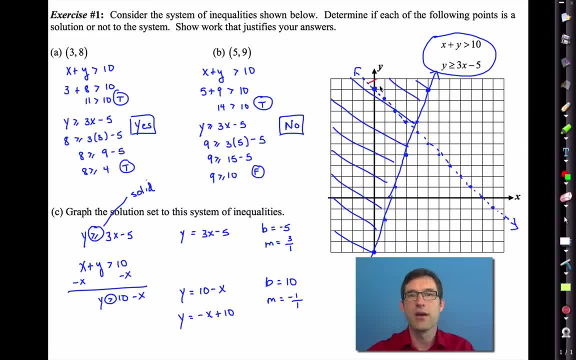 Y is greater than 10 minus x. so I'm going to shade above this line. Now, what exactly is my solution set? Well, remember, my solution set will be all the points that make both of these inequalities true, And that is going to be my solution set. 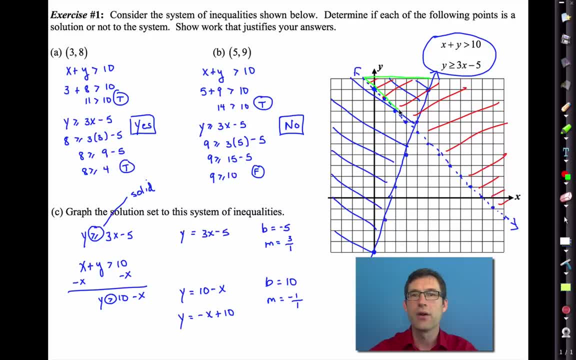 All right, So my solution set. I've already drawn this right here, right, So I'm going to draw this right here. The y is the outside of my solution set And the y is my solution set, And that's going to be my solution set. 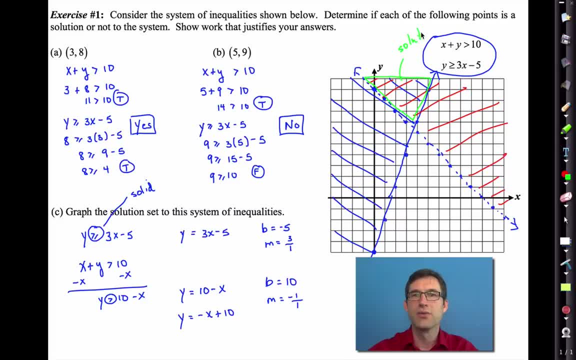 Okay, I'm going to use you guys to see how thisante's going to work. Okay, So this is my set And this is my solution set. This is my solution set. This is my solution set And, if you notice right, 1, 2, 3, 1, 2, 3,, 4, 5, 6,, 7, 8, there's my 3, 8, right. 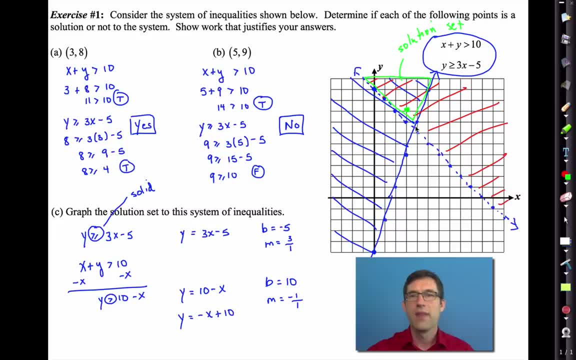 On the other hand, my 5,, 9,, 1,, 2,, 3,, 4,, 5 and 8,- this is the solution set Right- 4,, 5,, 1,, 2,, 3,, 4,, 5,, 6,, 7,, 8,, 9 is not in the solution set right. It's not in the double. 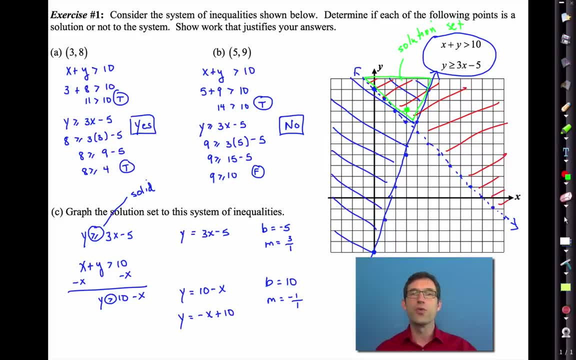 overlap. So the solution set to a system of inequalities is where the two parts of the shading overlap, if they overlap at all. right, But that's it. That's the whole story, okay, Okay, so pause the video. now Really think about what we did, because essentially we did. 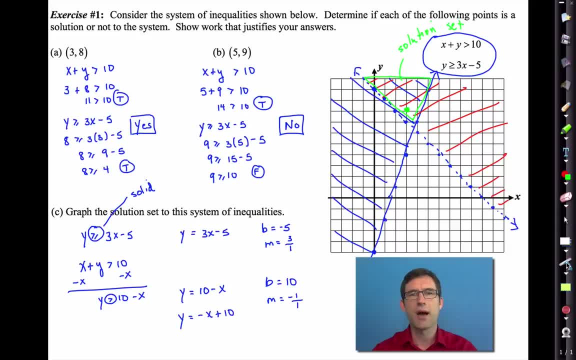 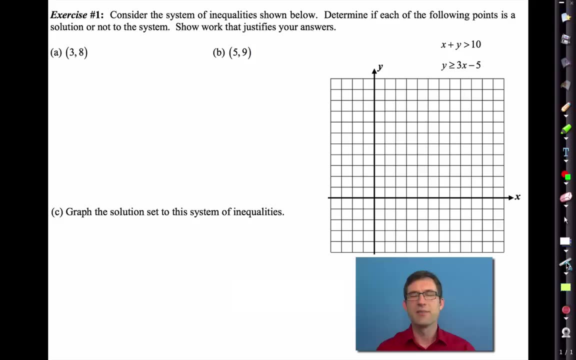 the whole lesson here We really did. It's just a combination of other things that we've done. I'm going to clear this out in a moment, though, so pause the video. All right, here we go. Okay, that's gone. Let's move on to the next exercise. So exercise number two. 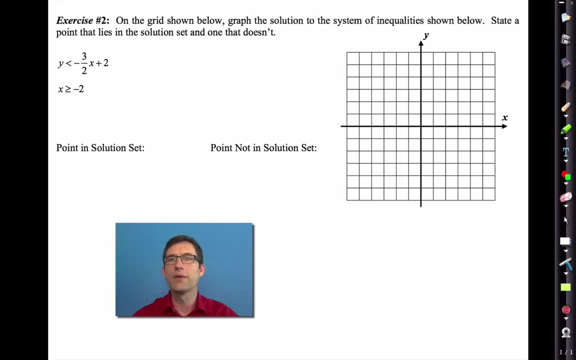 On the grid shown below graph: the solution set to the system of inequalities. The system of inequalities shown below State a point that lies in the solution set and one that doesn't. All right, well, let's start off with this guy, but maybe not in green. I mean we could. 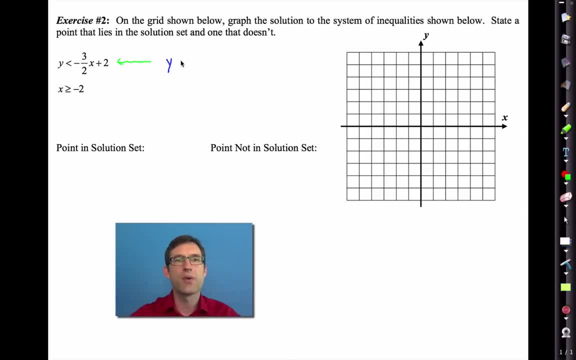 Now this one also already has y isolated, so I'm going to change it into an equation: y equals negative, three halves x plus two right, where clearly the y intercept is two and the slope is negative three divided. So that's going to be pretty easy to graph. I'll do that. Go down three to the right two. 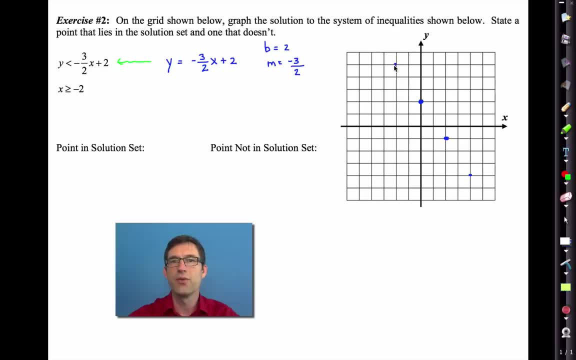 Reverse it, Go to the left, three up, two, All right should be dashed, right Dashed because there is no equality there. so the points along that line are not included. The boundary points are not part of the solution. That's why we dash it, And then I think I'll do. 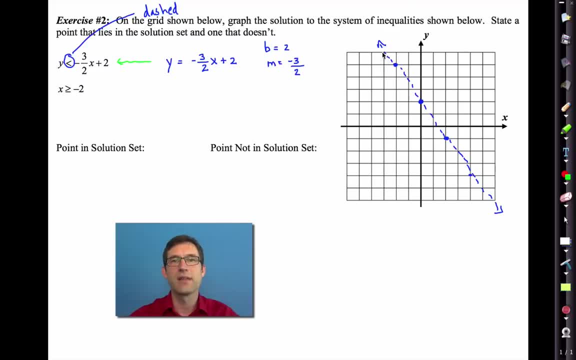 the shading right away. We're supposed to be doing the shading right away, but we're supposed to be shade under it because it's less than So. any point in there, and I think I'll label the equation of the line. y equals negative three halves x plus two. All right, let me change colors. 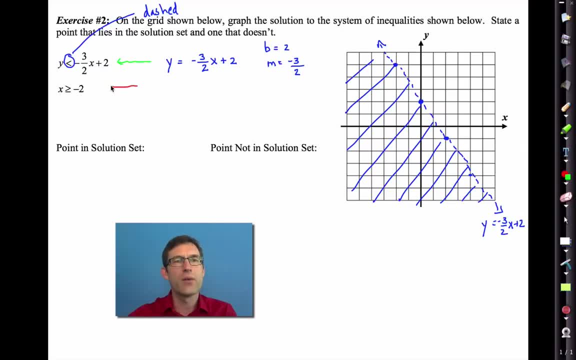 We go to red. now for the next one. Now, what do we do with this guy? Well, the line it's based on is x equals negative two, All right, but that is a vertical line, right, It's the line that has all x coordinates of negative two. 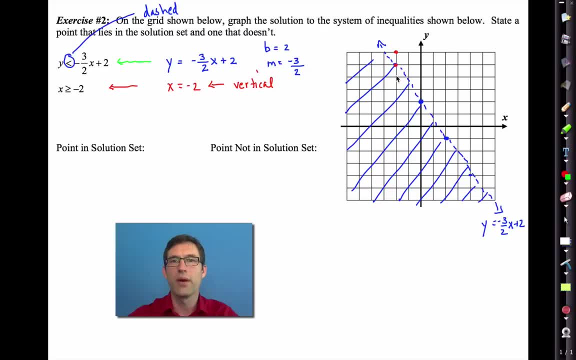 So, for instance, that point's got an x coordinate of negative two, and that point and that point and that point- right, It's all points that have x coordinates of negative two, All right, and it should be solid because the equality is included. 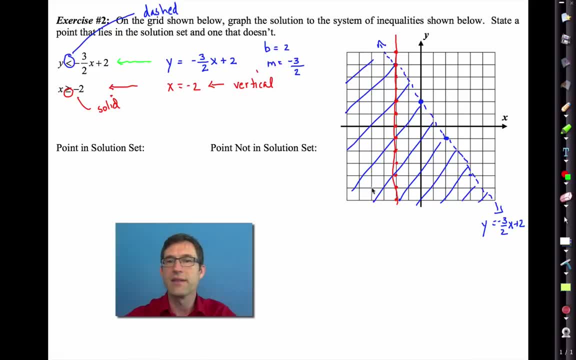 So I'm going to draw a nice solid red line As well, as I can not all that great Label it. x equals negative two, and now it's greater than Now. that's a little weird. right, Because it's not above or below. It's right, left. 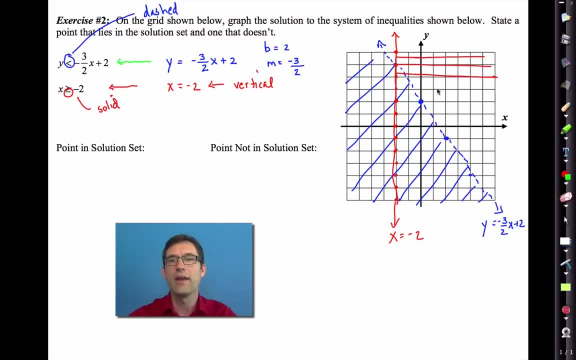 and of course, greater than in this case is going to mean to the right, because all x coordinates to the right of negative two are greater than it. Okay, so that's it. I mean that's the whole deal. Now what's interesting is, again, the solution set itself is sort of this: 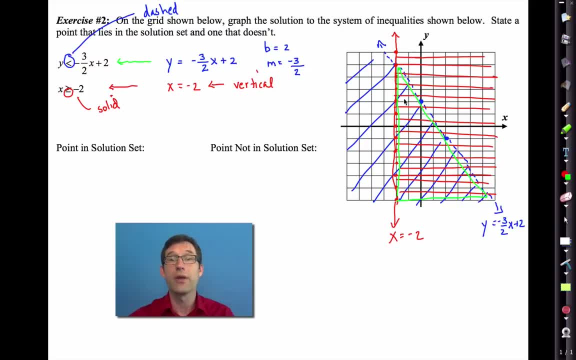 overlapping region, which includes this boundary but doesn't include that one. So the last part of the problem says: give one point that's in the solution set. Well, there's tons of points, tons of them. Here's a really good example: Here's a point that's in the solution set and that's got the coordinates negative. one one. 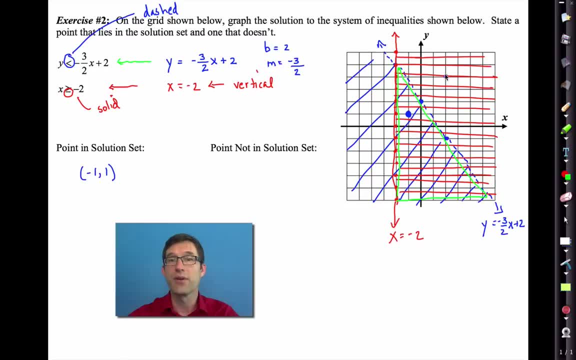 On the other hand, there's also lots of points that aren't in the solution set. For instance, this point is not in the solution set and it's at one: two, one, two, three, four. But that's it. That's the whole deal. 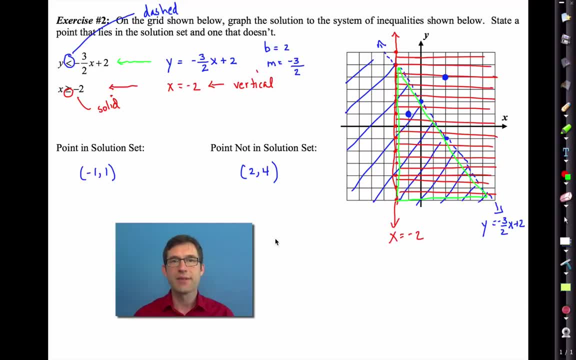 So graph the lines that the inequalities are based on: shade according to greater than or less than and wherever the shading overlaps of the two inequalities, if at all. that is your solution- set. Okay, pause the video now and I'm going to clear out the text. 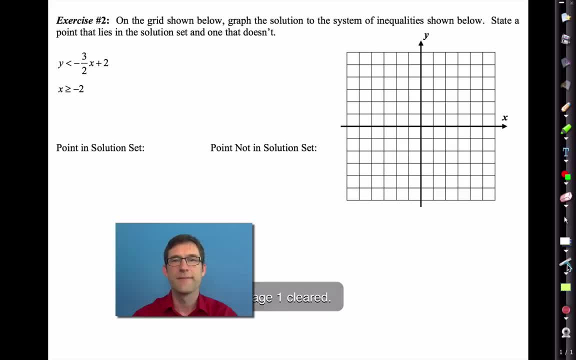 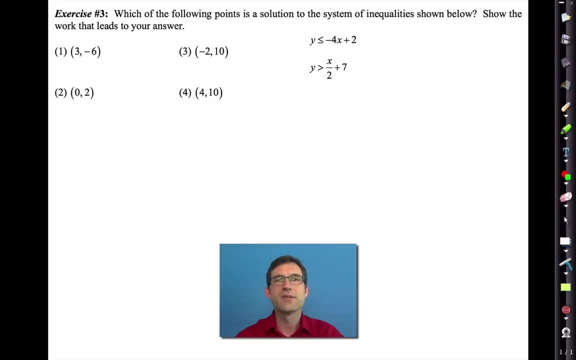 Here it goes, All right. Exercise three: Nice little multiple-choice problem. Which of the following points is the solution to the system of inequalities shown below? Show the work that leads to your answer. Well, we have no graph paper here. All right, if we had a piece of graph paper. 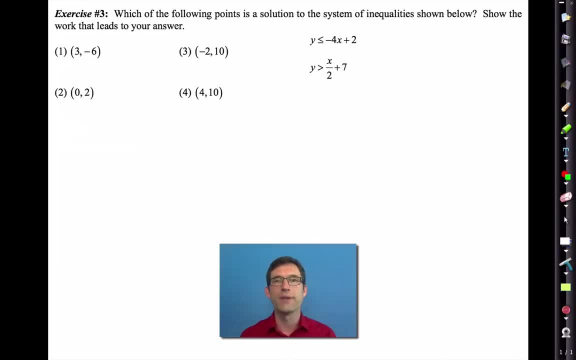 we could do the full-on problem, graph it all and then simply plot the four points. But here, Here, we really have to rely on truth values, and it's kind of annoying, it's kind of a guess and check thing. but remember, if either one of the two are false, then the whole thing. 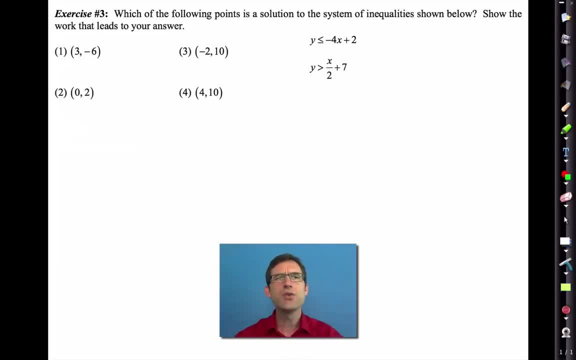 is false, okay, So let's do one. let's walk through one that is false and then have you work to find the one. that's true, okay, So let's try number one. okay, the three comma negative six- Let's try. y- is less than or equal to negative four x plus two, so I'll put negative six. 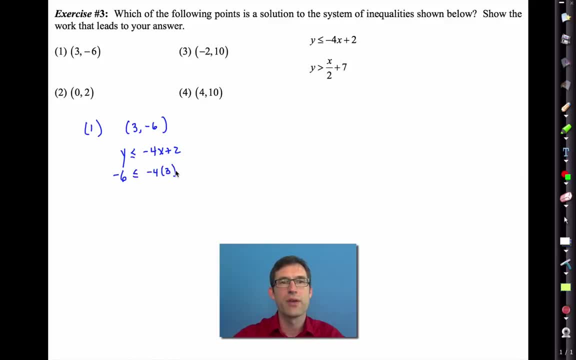 in there, less than or equal to negative four times three plus two. negative six is less than or equal to negative twelve plus two negative six is less than or equal to negative ten. Well, that's actually false, right? Negative six is greater than negative ten. 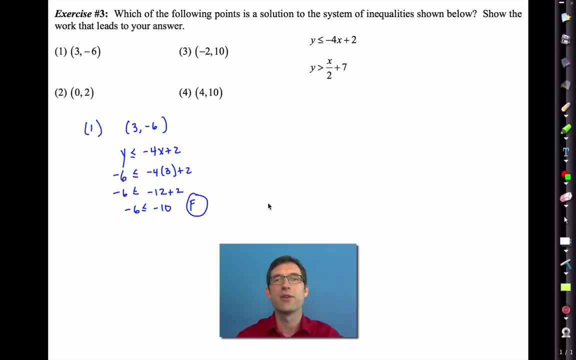 Remember that if you struggle with comparing two negative numbers, think about them in terms of temperature. Which one is warmer? Negative one? right, They're both cold, but negative six is warmer than negative ten. So that's a false statement, which means I don't need to do any more work on number one. 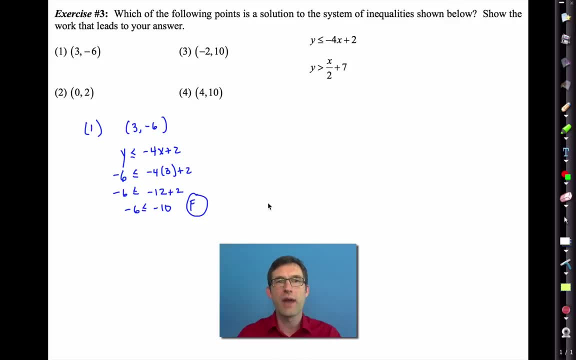 it can't be a solution to the system, So pause the video. now work through your other three choices and see which one makes both of those inequalities true. Alright, let's go through it. The correct choice here actually ends up being choice three. okay. 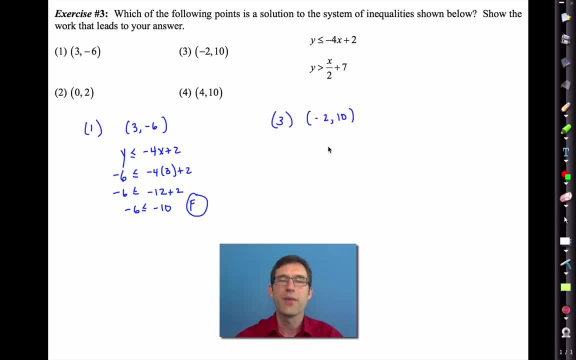 And let's work through it really quick. So choice three is negative two comma ten. Alright, here we've got y is less than or equal to negative four. x plus two. If I put ten in right, I get negative four times negative two plus two, negative four. 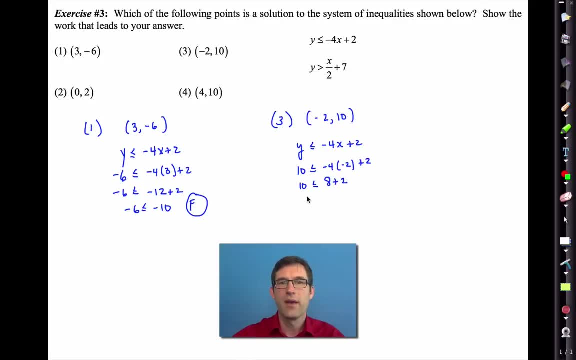 times negative, two and negative times. a negative is a positive and I get ten is less than or equal to ten. Had that just been a less than, the answer would have been false. but because there's that equal there, it's true. 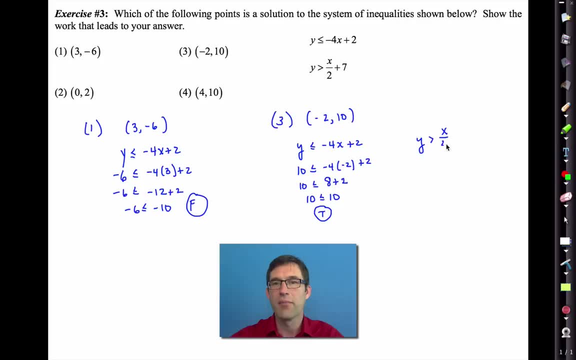 Likewise, let's check this: one x greater than x divided by two plus seven. whoops, let's put in the ten for y greater than negative. two divided by two plus seven. negative divided by a positive is a negative and negative. one plus seven is positive six, and that's also true. 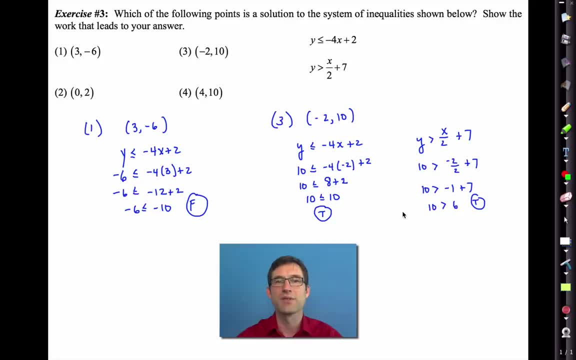 So since both inequalities are true, at that point it is part of the solution set. The other two choices either fail in both cases, Alright. here we go. Both of the inequalities, or fail in at least one, Alright. so pause the video now. write down anything you need to. 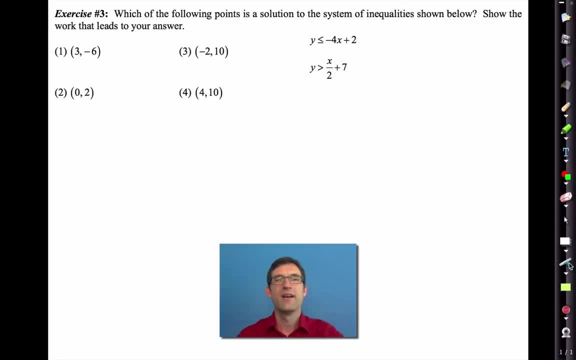 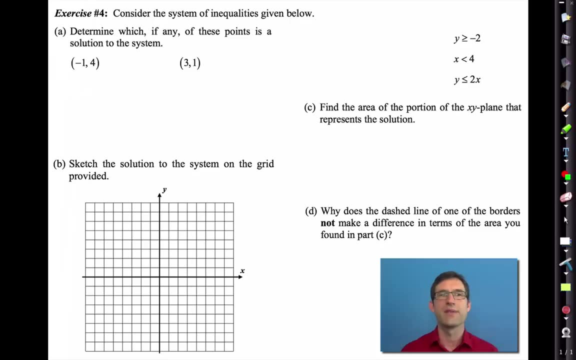 Alright, here we go. Let's move on to the last problem, Exercise four. I like this one a lot. Consider the system of inequalities given below. Determine which, if any of these points, is a solution to the system. So I've got these two points and I want to know: are they solutions to this system? 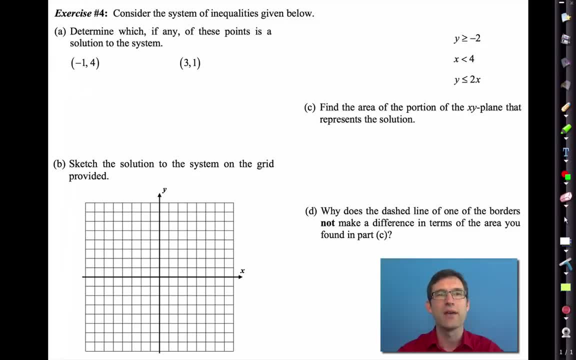 And I know it's now three inequalities. That's okay, We'll live with them. Two of them are very, very simple. So check, pause the video now and see if either one of those points is a solution to that system. Remember, all three have to be true. 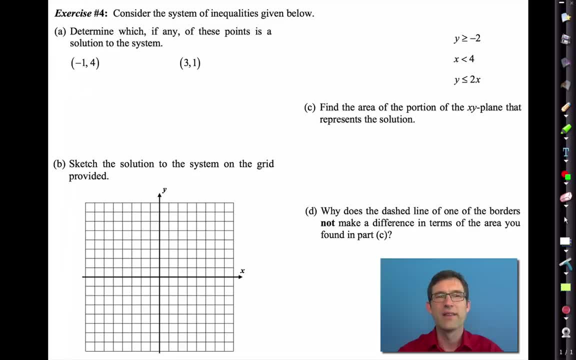 Alright, let's go through it. Well, let's check them one at a time. This inequality, y is greater than or equal to negative two. Well, is four? Is four greater than or equal to negative two? Yeah, that's true. 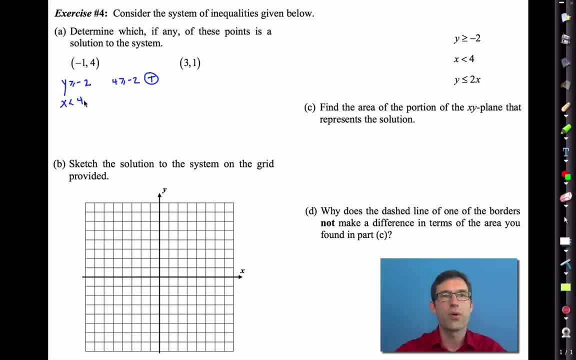 One down. Our next one is: x is less than four. Well, is negative one less than four? You bet it is, That's true. Our last one is: y is less than or equal to two. x- That will be four- is less than or equal to two times negative. one or four is less than. 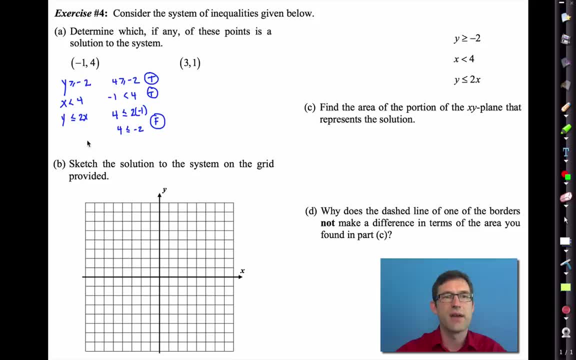 or equal to negative two. That's a false and therefore no, Ah, came so close. two out of the three. Alright, let's try this one. So y is greater than or equal to negative two. Well, that would be. one is greater than or equal to negative two, and that's true. 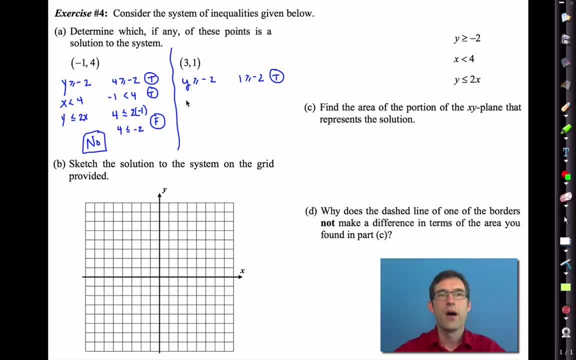 Right, because one is bigger than negative two. Alright, then we have: x is less than four, That's. three is less than four, That's certainly true. And y is less than or equal to two. x- That would give me one- is less than or equal to. 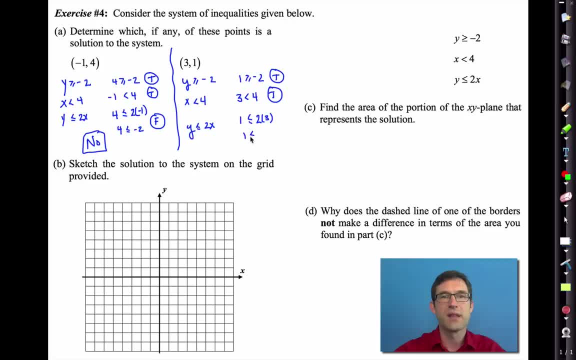 two times three, or one is less than or equal to six, and that's certainly true. So, yes, So, when I eventually am asked to graph this thing, well, we know that the first point won't be in the solution and the second will. 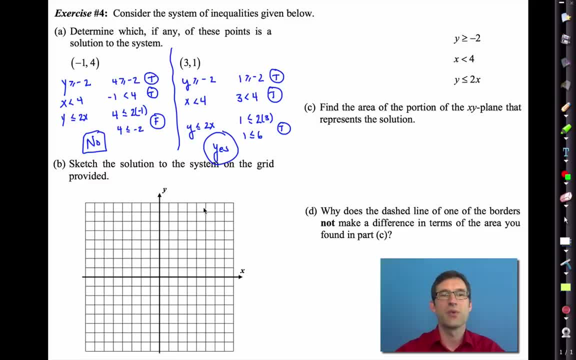 So let's do it. I'm going to do some of the writing up here as we graph it down here. But y is greater than or equal to two. We'll do that. one in blue. That's going to be based on this horizontal line, right? 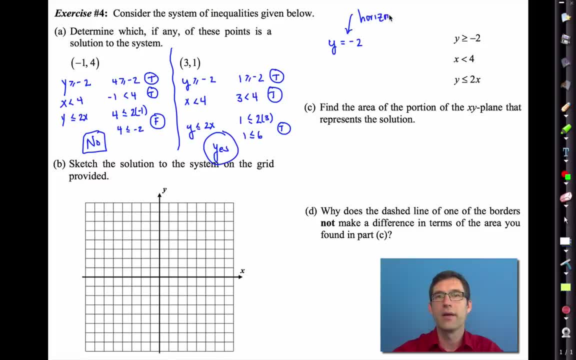 Horizontal line. It's the line where all y-coordinates are negative two. So, for instance, this point, this point, this point, etc. right, I don't think I really have to draw them all out, But every single point along that line has a y-coordinate of negative two. 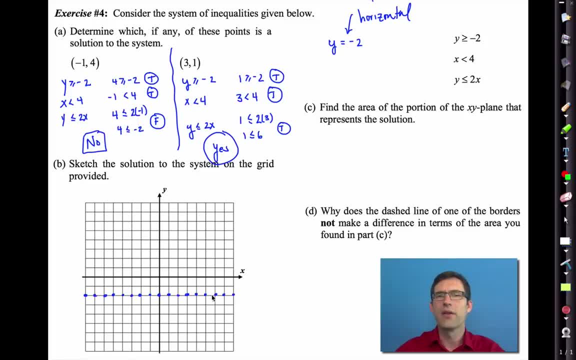 And yet here I am doing them all: Alright, solid or dashed. Looks like it should be solid because the equality is included And greater than means that we should shade up Here. Alright y is equal to negative two. I keep forgetting to label my lines. 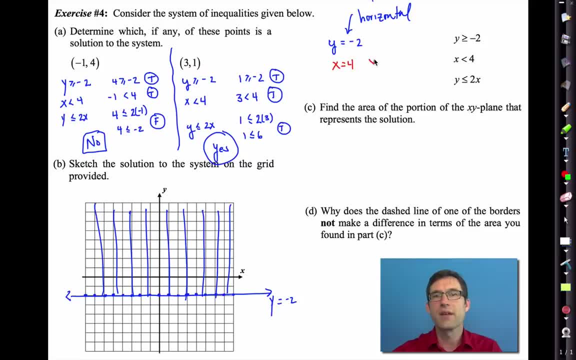 Alright, let's do the next one. x equals four. That's going to be vertical Right, And that's one, two, three, four. Any point along this line right has an x-coordinate of four, Right, Solid or dashed. 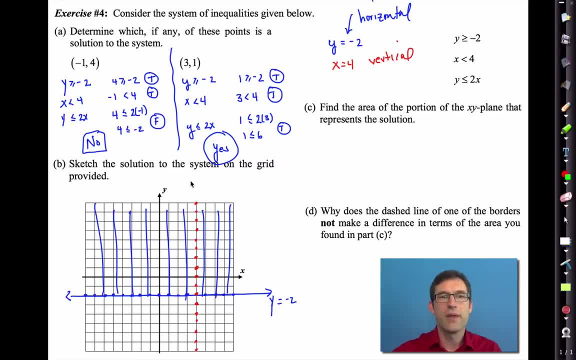 Well, it's just less than So. that seems like it's dashed Right. That's definitely dashed Okay, and let's see It's less than So. this is going to get to be a little bit of a complicated picture. 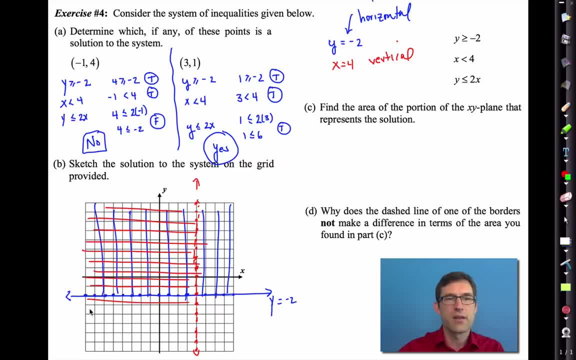 But that means we've got a shade to the left. There we go, And let me go to the last one in green. Here we'll go with: y is equal to two x. Now, this one's interesting, Because this is definitely a slanted line. 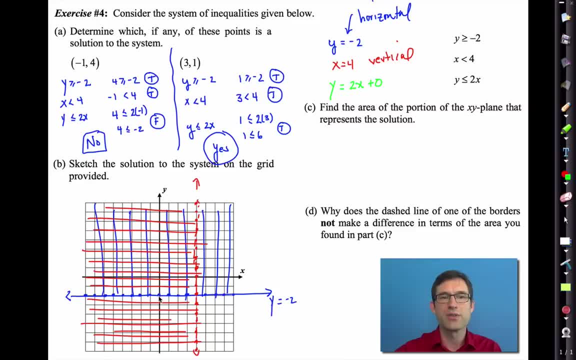 Right, Both the x and the y are there. I put that plus zero in just for us to be able to think about the y-intercept of being zero And a slope of being whoops. that's not a y-intercept of zero. 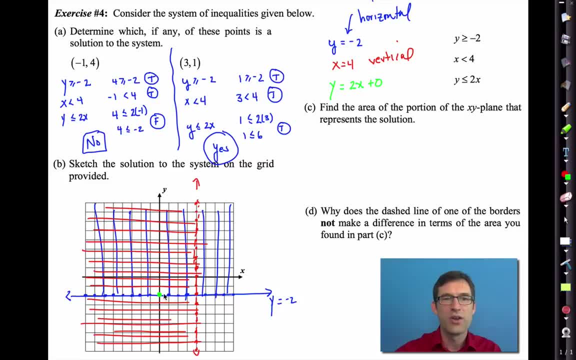 Oh, this is going to be tough to erase. I've got to go super duper small. There we go. That worked. There's my y-intercept of zero, And then I'm going to go up two and over one. 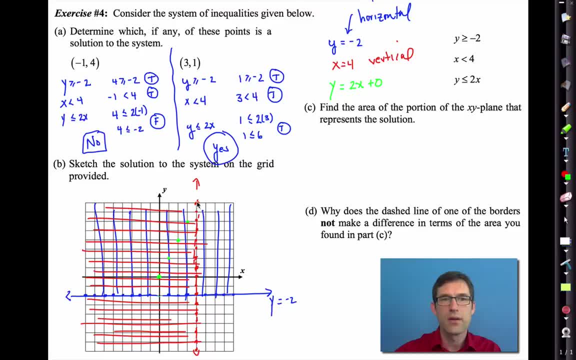 Up two and over one. Sorry about how messy the picture is getting, But we do have three boundaries on there. All right, Solid line, Because Let me go back to red and label that other line. X equals four. Now go back to green and do some shading. 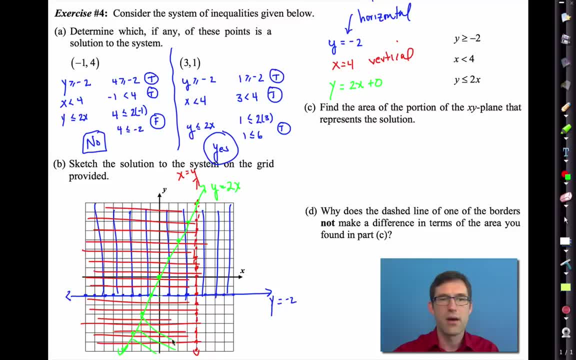 That's going to be less than So, it's going to be under that line. Ooh, So where in the world is my solution set? Let me outline it in black Right: It's wherever the shading crosses each other. 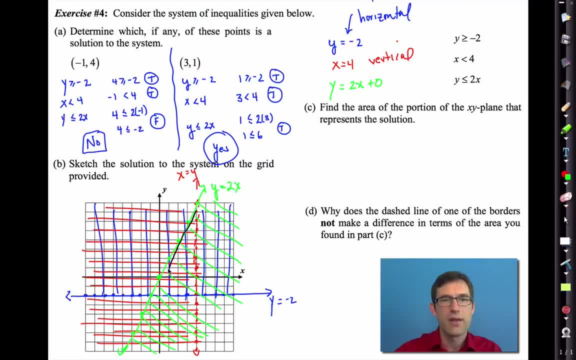 Right, All of them together. That's all in here, Over to here And down to here Right. Everything in here is the solution set, Everything in there. Now, letter C asks us to find the area of the portion of the xy plane that represents 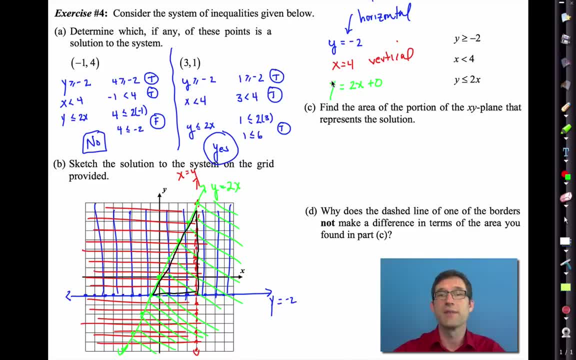 the solution. Well, let me pull that little puppy out. It's a nice right triangle. We can figure out its base: One, two, three, four, five. Figure out its height: One, two, three, four, five. 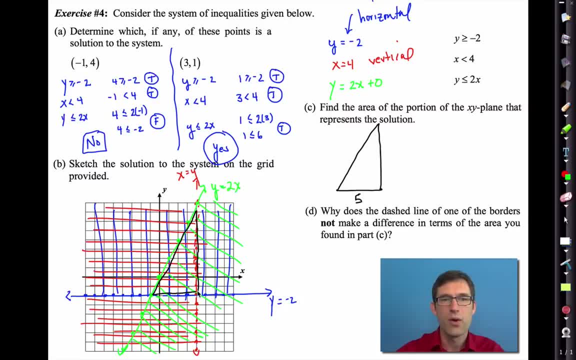 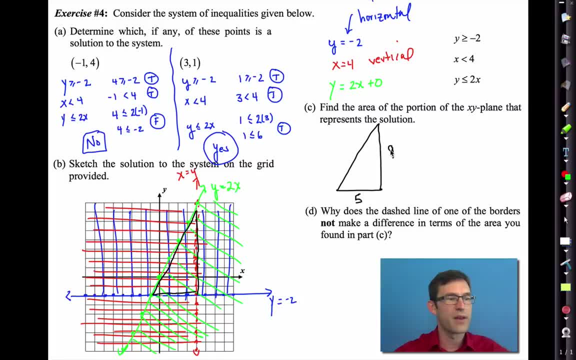 Nine or ten? Oh no, We're all the way up to here. All the way up to here. That was my mistake. Sorry about that. Yeah, The solution set extends all the way up there, So it's not nine. 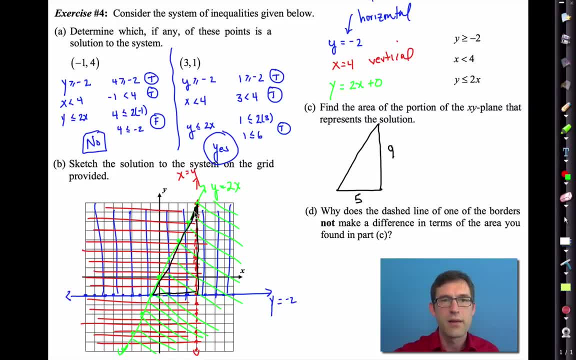 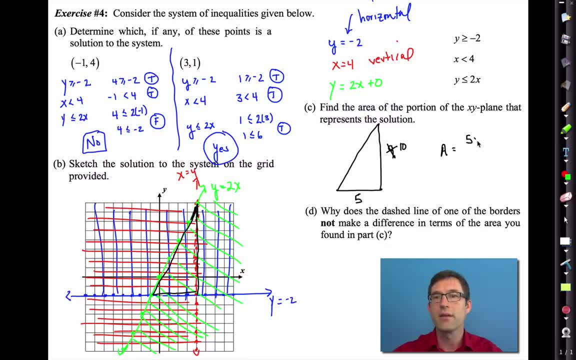 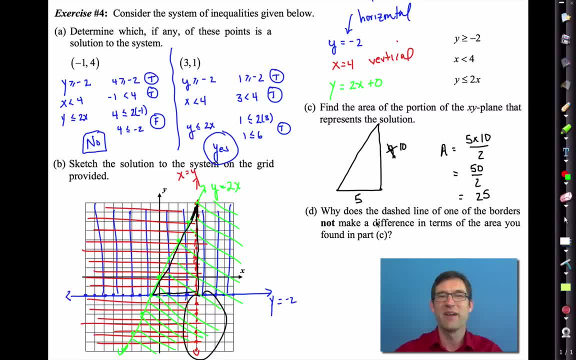 of one of the borders, and that's this border. my x equals four border. why does that make no difference in terms of the area? All right, Think about that for a second. This is actually a little bit of a tricky question. 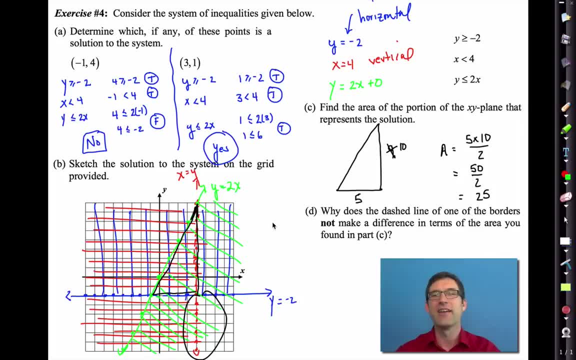 I just dropped my pen. Think about why the dashed line doesn't make a difference. All right, Pause the video now. Okay, I'm going to retrieve my pen, Oh, and I'm back. Hey, Hi, Okay. So here's the reason. 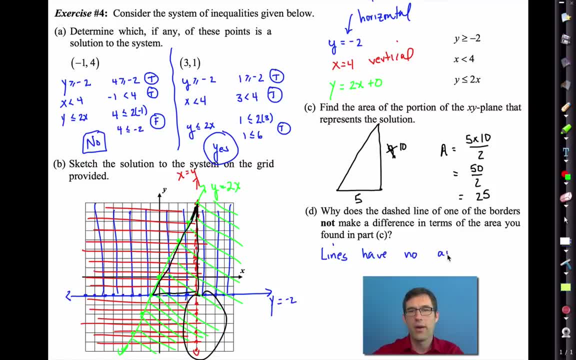 Lines have no area. So, in other words, the dashed nature of that line doesn't affect how much space it has, is within the figure, Doesn't affect it whatsoever. All right, In fact right, because the lines have no area, all three of the borders could have been dashed. 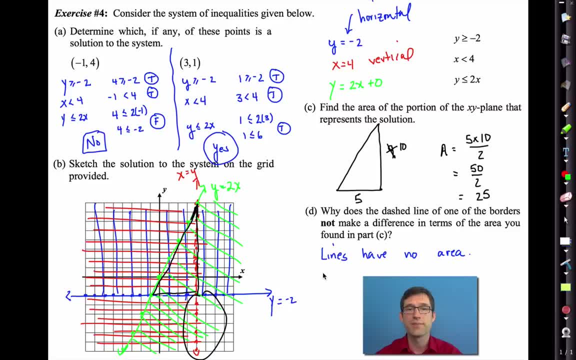 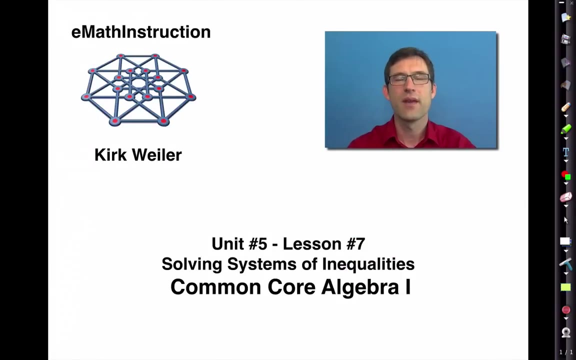 and the area that was shaded would have still been 25 units. Okay, so there's a lot on this page, lots of colors. I'm gonna clear out the text pretty soon, so pause the video now. All right, here we go. Let's finish up the lesson. So today, what we did is we